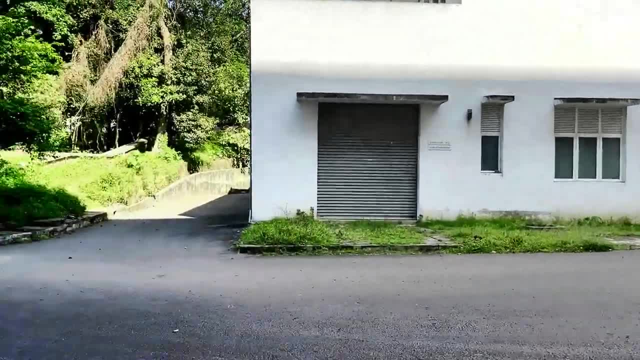 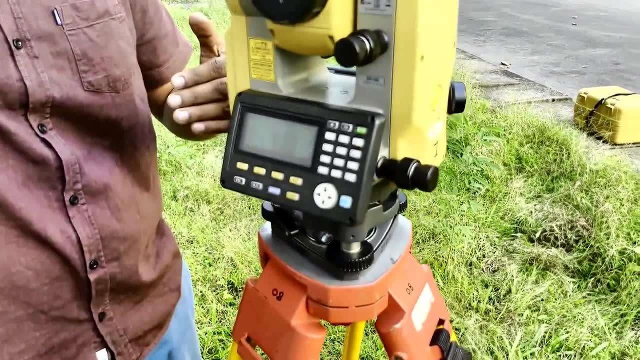 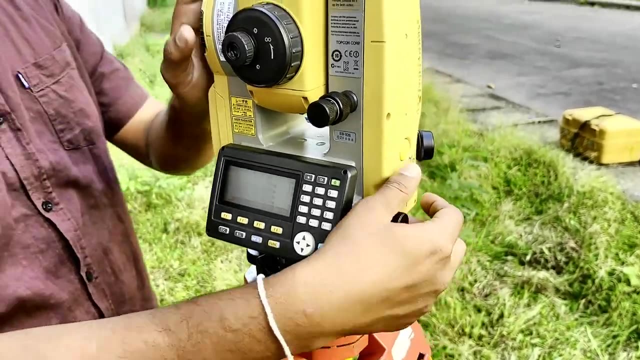 to 9,012 from 9,011.. So this is the instrument. So this instrument has been set up above the 9,011.. So we are going to measure the clockwise angle, that part of the instrument, right. So first I need to make it facelift, like: 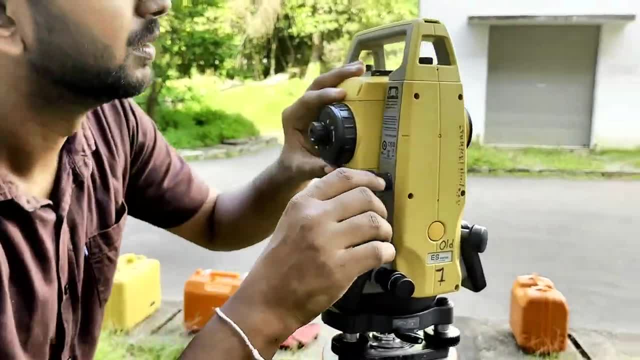 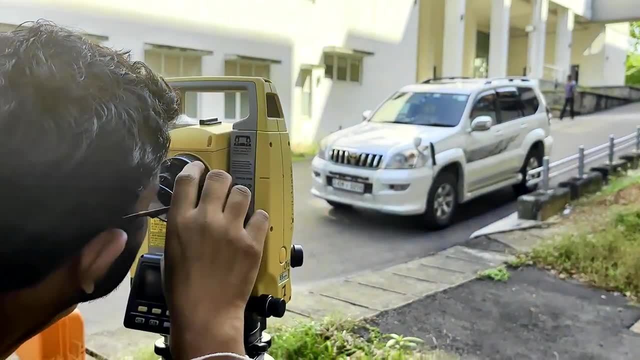 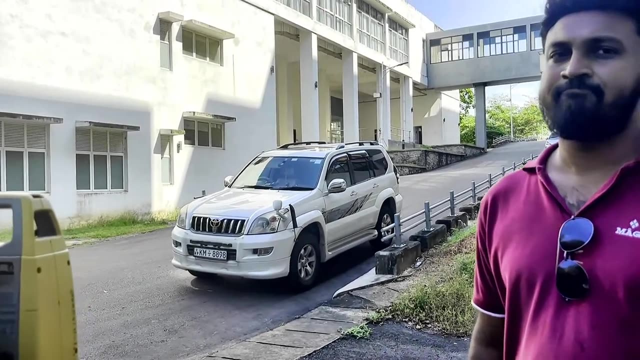 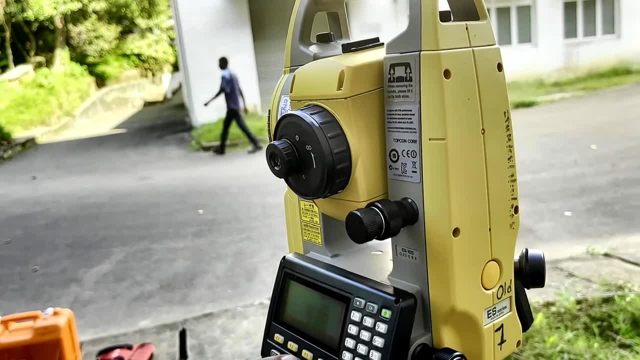 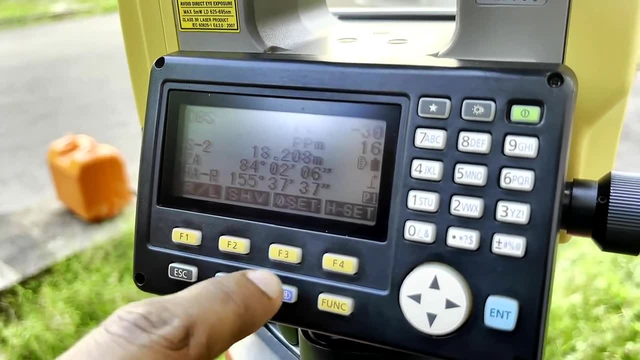 I need to correct it from the focusing screw Now. it is fine. Now I need to go to again. I need to see the angles. For that I go to SHC mode back Right. So when I see the SHC mode I can see the HA-R is 155,, 37,, 37, like that. 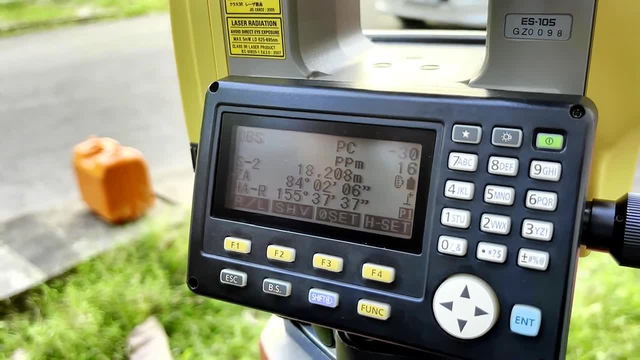 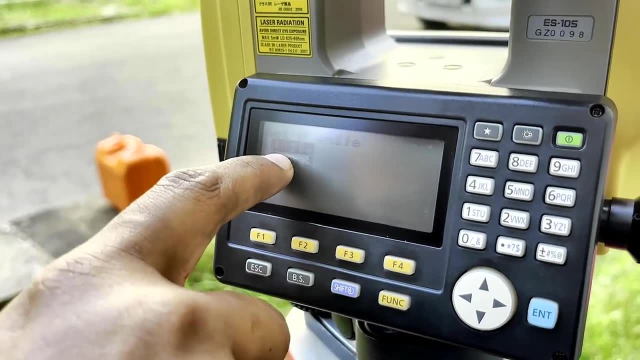 So if I need to give a predefined angle to the facelift of this camera, this line right. so i go to hset. if i go to hset, there is one option called angle and other one is called coordinate. so we go to angle, so i give the predefined angle here. 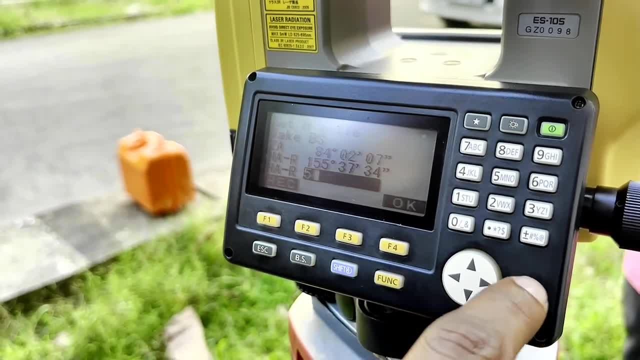 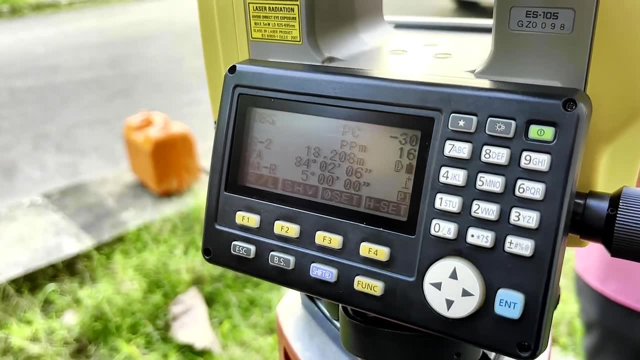 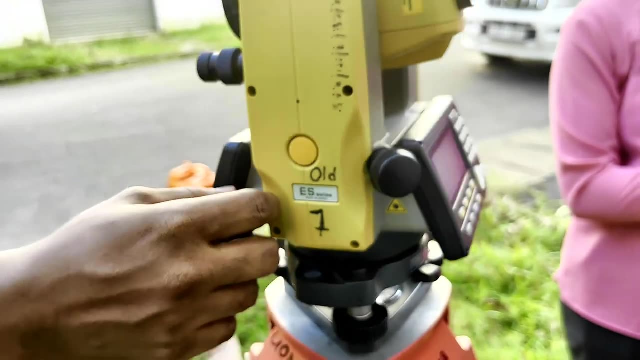 so i i like to give five right five for this one. so i i click five, press five and click. okay. now the angle i have given for that station is five right. so now i am going to turn the instrument clockwise like this, clockwise in phase: the population i'm going to target. 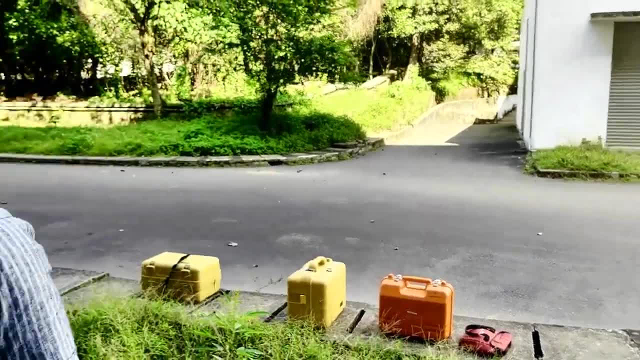 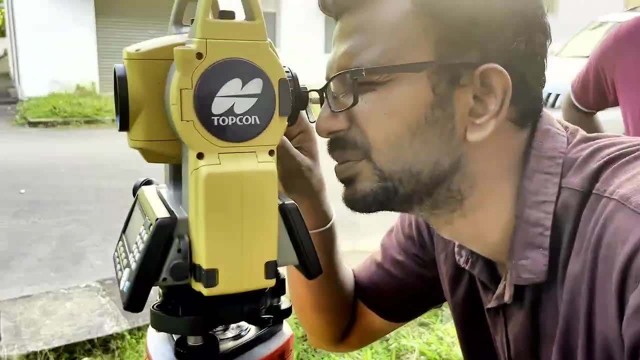 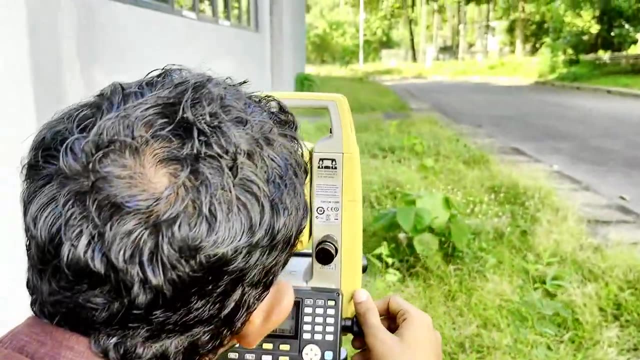 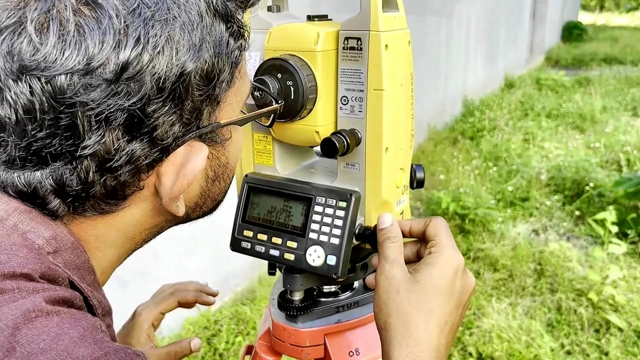 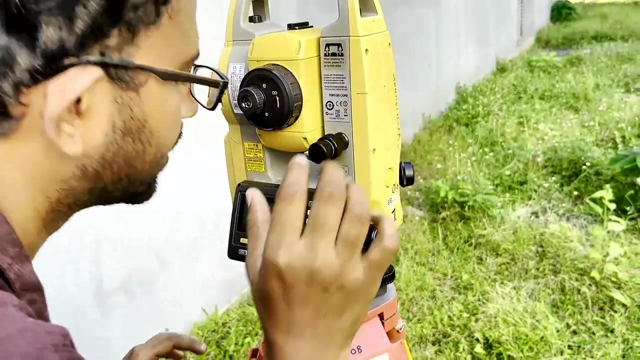 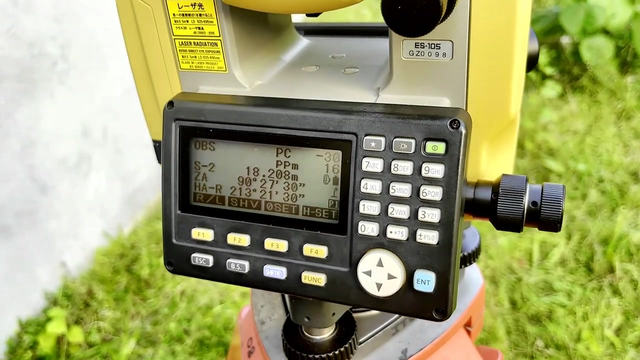 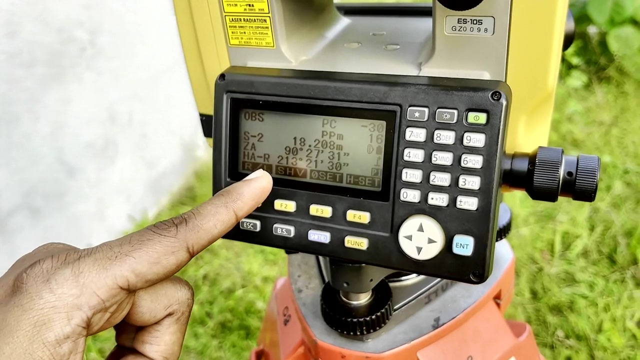 see that that one nine thousand quid right now. you can record the angle. it is 2, 13, 21, 30, right. anybody can record the angle: 2, 13, 21, 30. that is the face, yes, first right face left angle to 9000, 11, 9000, 12, line right. 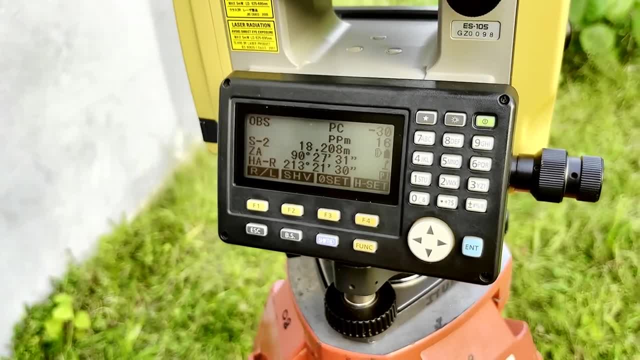 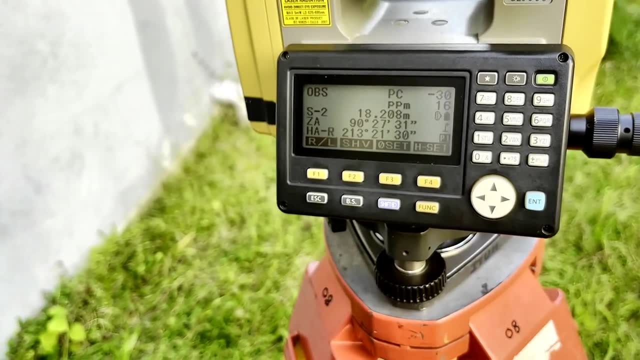 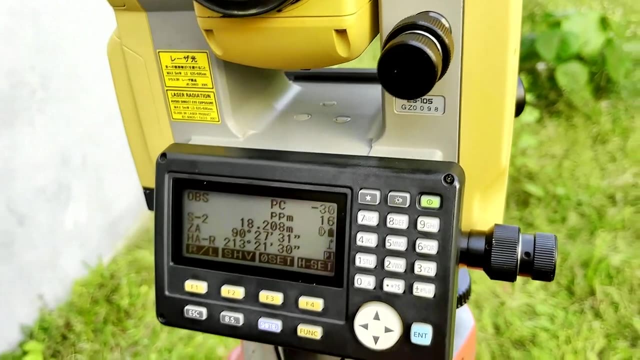 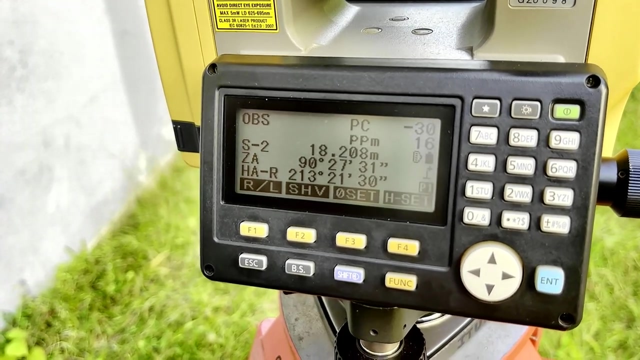 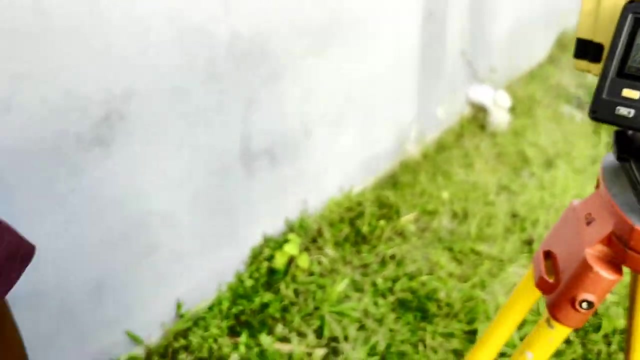 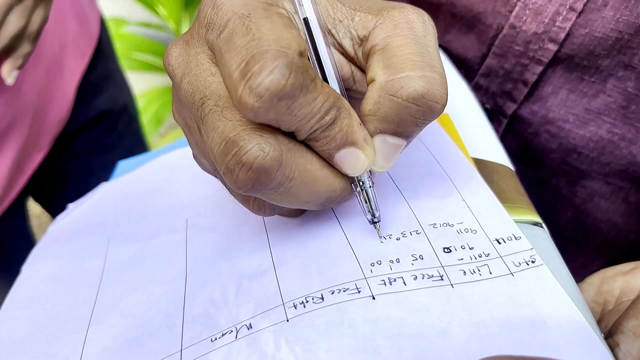 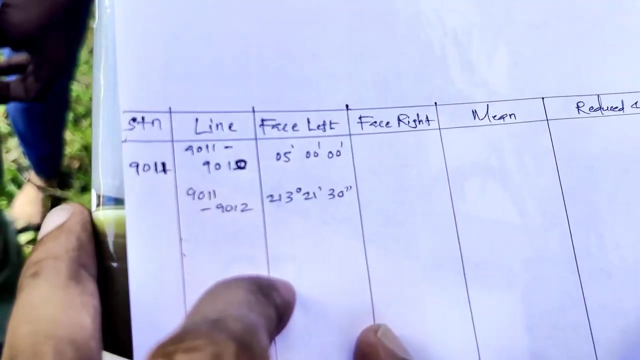 then, oh right, it is 2, 13, 21, 30 seconds. right, the first one is five. put it as five. this is nine thousand ten. right. that line, that line, 9000, 11, 9000, 12 line. it is 2, 13, 21, 21, 30 seconds. right. these are the two face left angles. 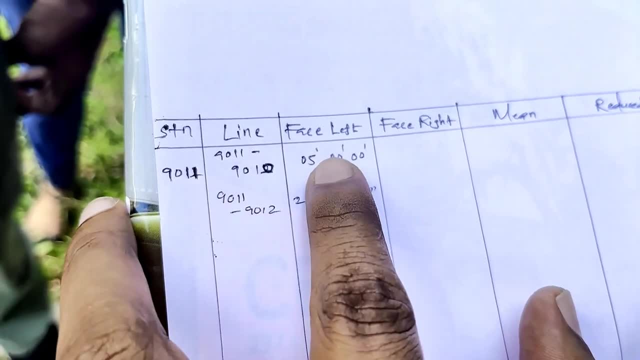 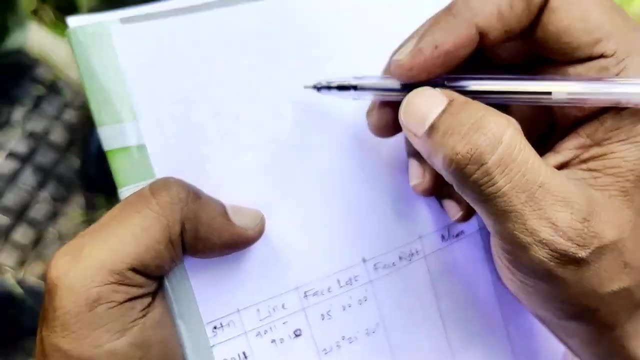 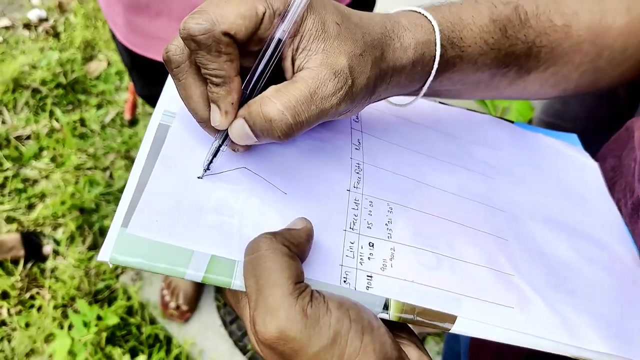 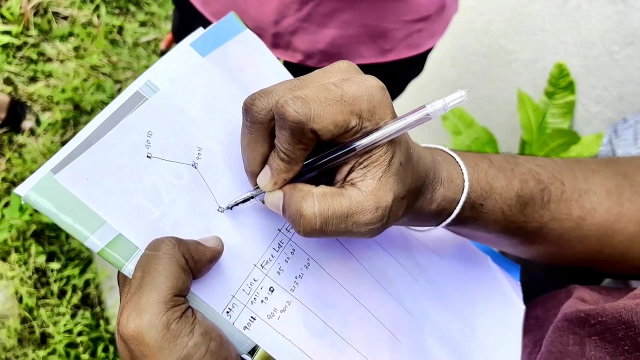 we obtain from four 9000 11, 9000 10 line. this is five 9000 9000 12 line. right? so if i draw it like this: this is 9000 10, this is 9000 11, this is 9000 12. here we have observed five. 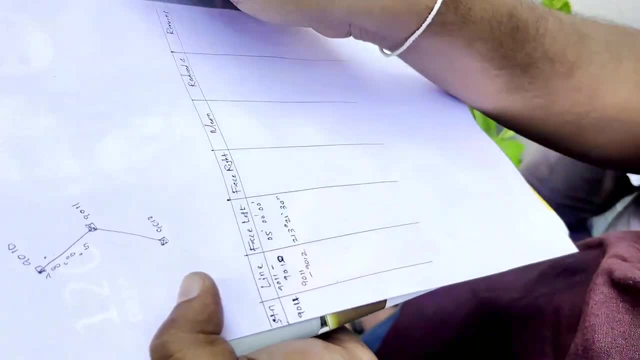 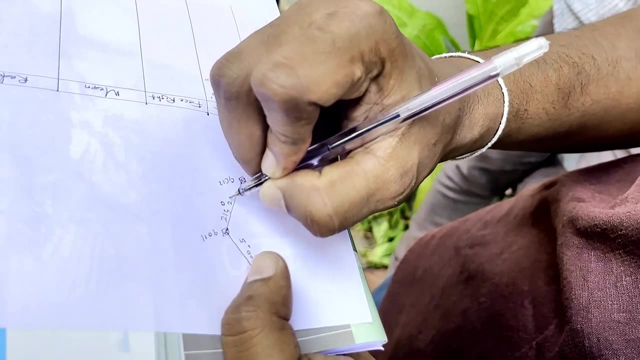 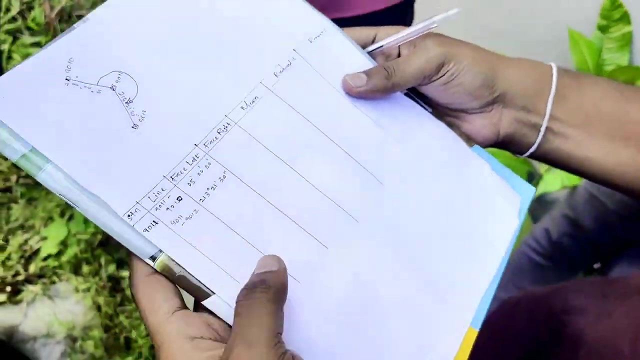 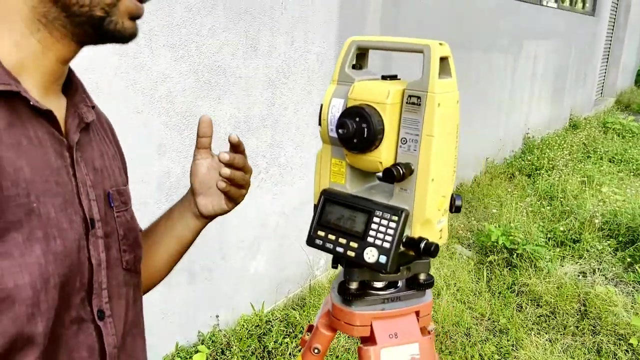 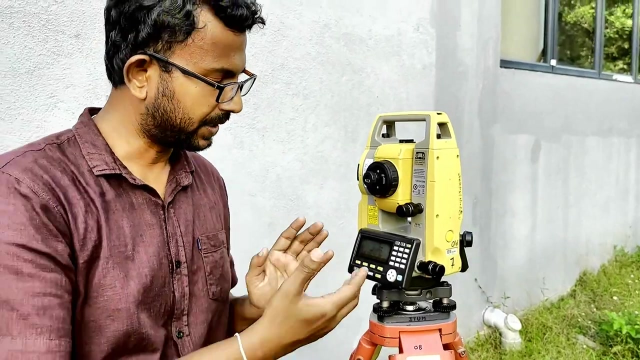 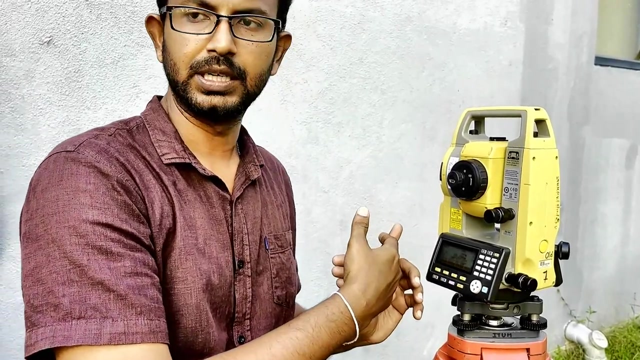 here we have observed 230, 21, 30. right, some get the right reading right. how we are going to get the phase right? you know that angle reading increases when this upper plate- upper plate- is turning about the instrument axis. right now the upper plate is not turning. right now the upper plate is not right. in that case the angle is not. 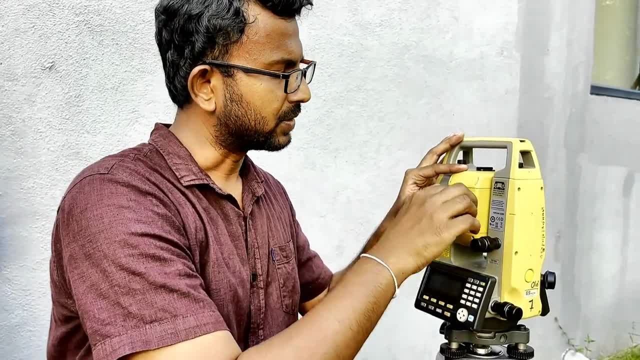 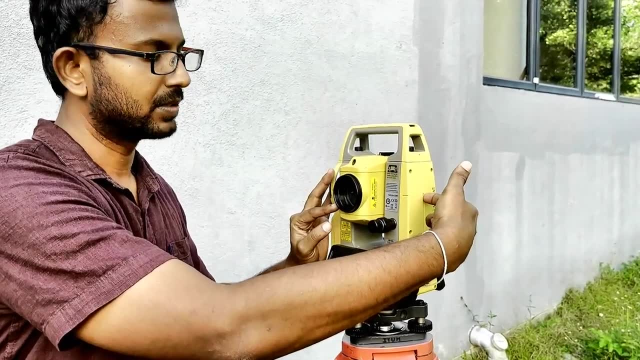 going to change, rightativamed, a particular whoever is getting a movement around, so on, But the direction is going to change by 180 because we are going to turn for the transit of the telescope about Trunian nexus. So now I have transited it. So now the difference between that direction and this direction is 180.. 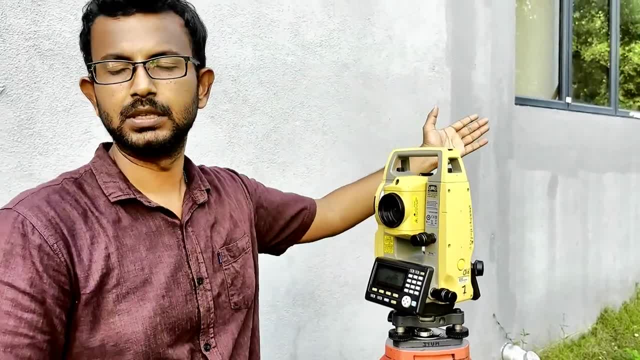 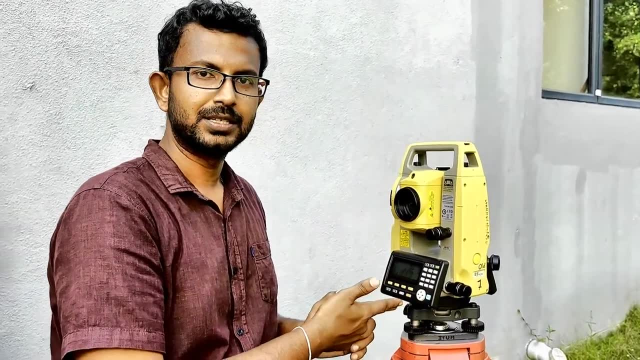 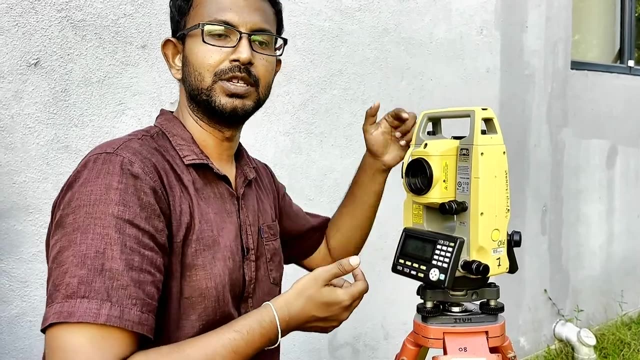 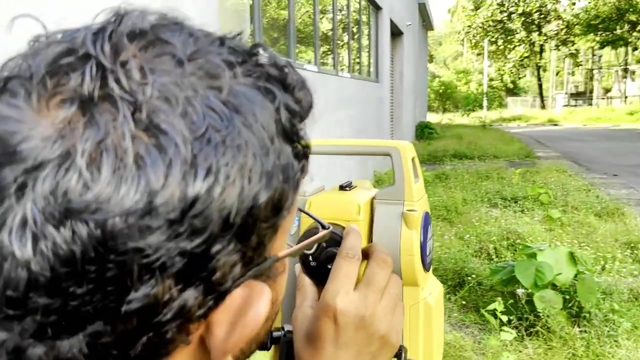 Therefore, if I need to target back to the 9012, I need to turn the instrument by 180.. When I am turning the instrument 180, now it registers the turning angle because the upper plate is turning about the instrument axis. So I am turning it and clamping screws. 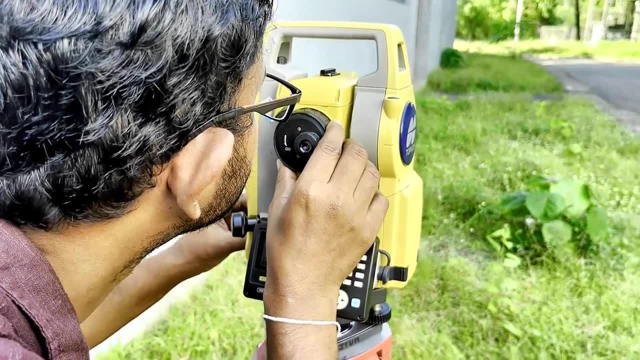 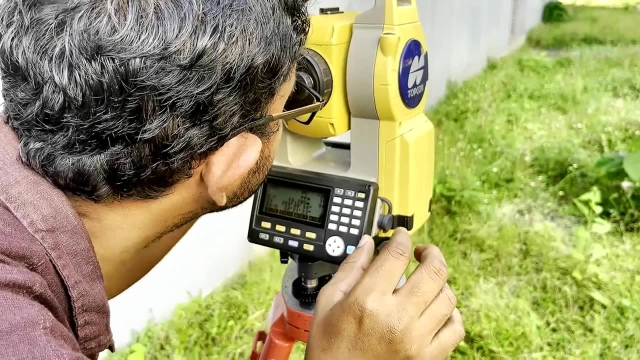 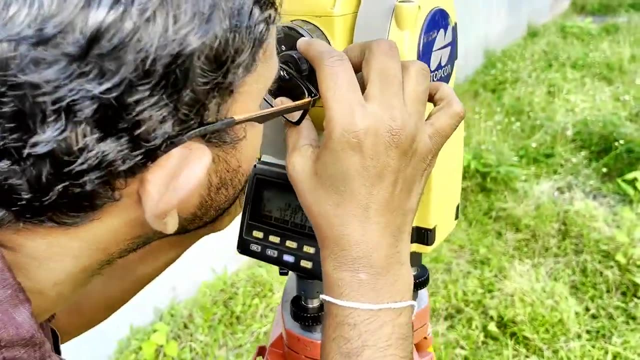 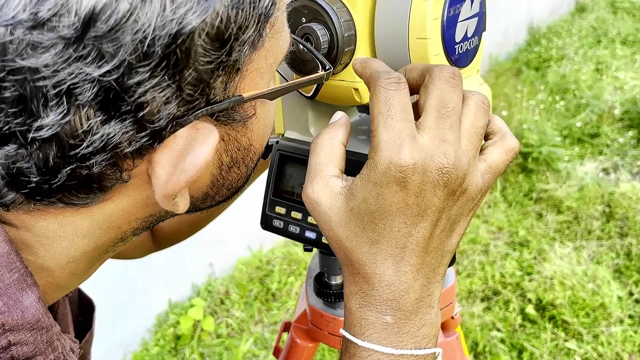 I am turning it and am interrogating whether it ministers to me or to adherents. I am able to find my instrument because I am umbilic Cambodiaитанus, Itssta in this direction. Here there is my instrument, Itssta. This is out here. 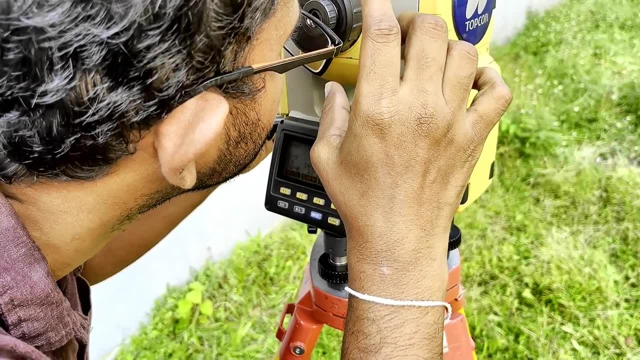 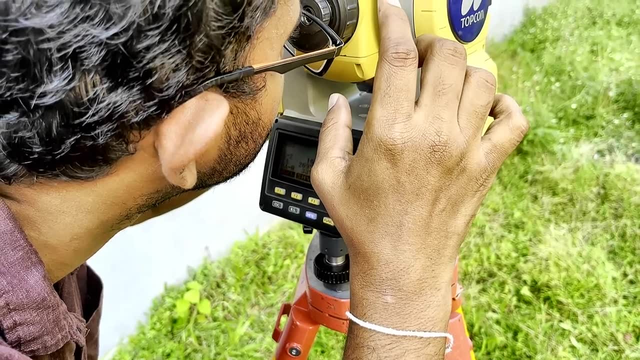 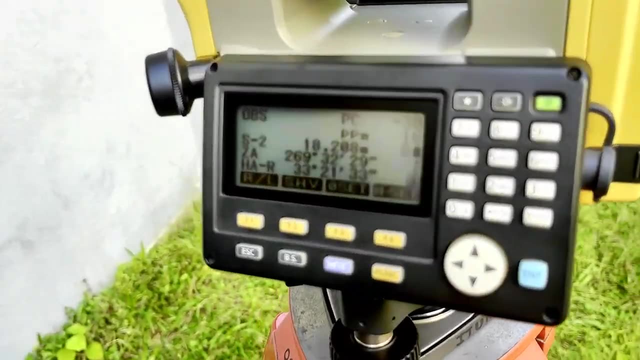 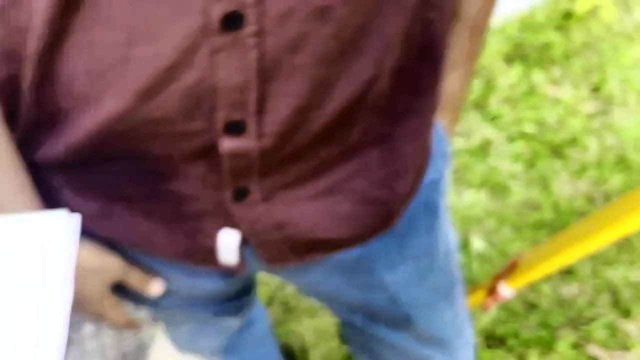 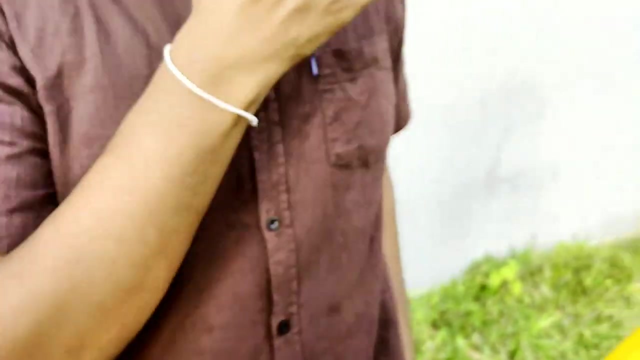 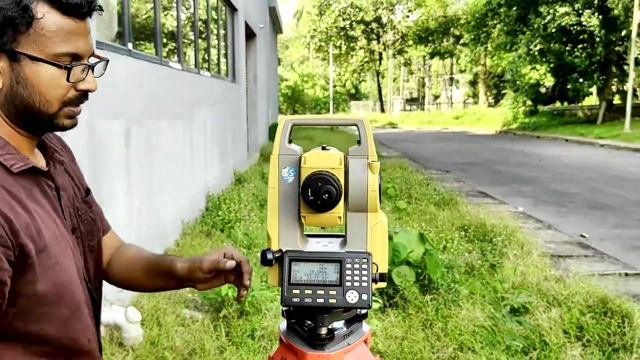 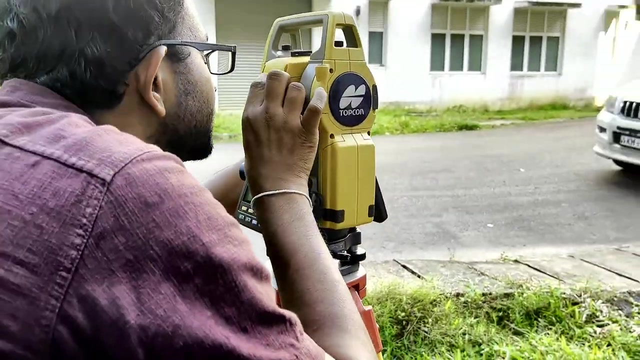 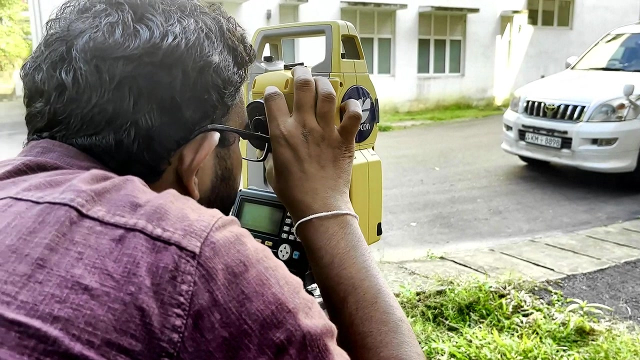 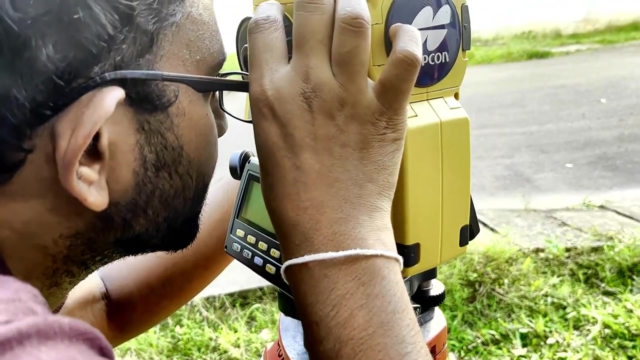 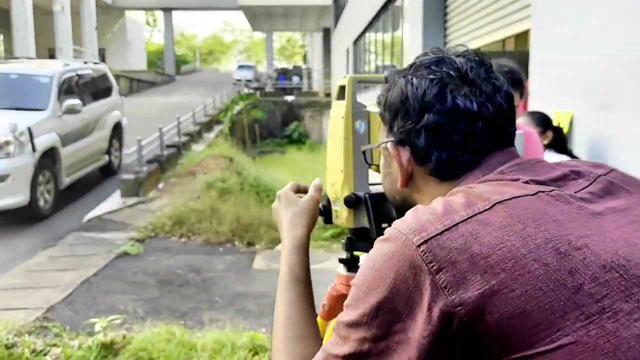 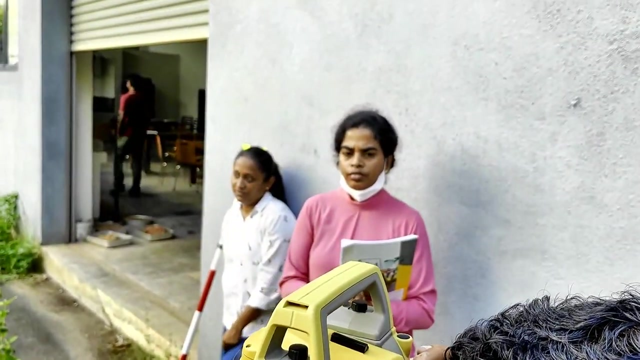 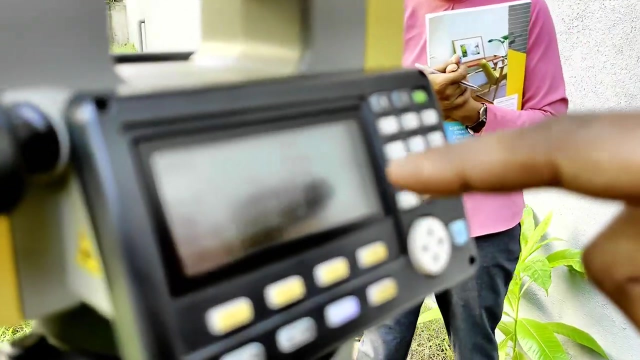 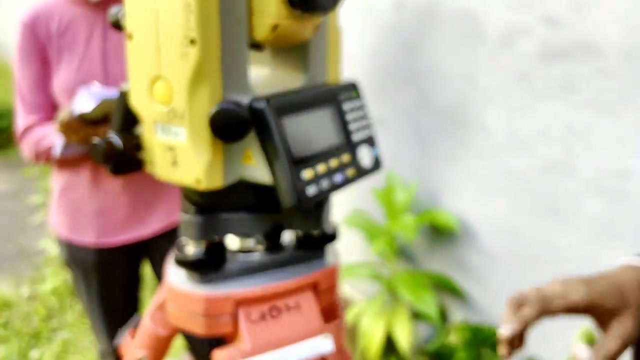 right, it is 33 21 33, 33, 21 33. yes, right now we need to get the face right reading of 9000. so it is 185, 0 minutes and 4 seconds. now you see how close it is right if the 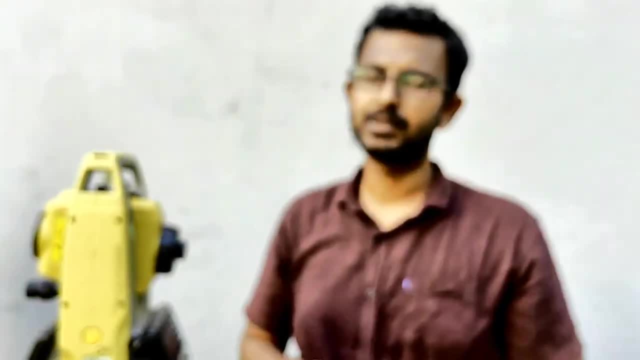 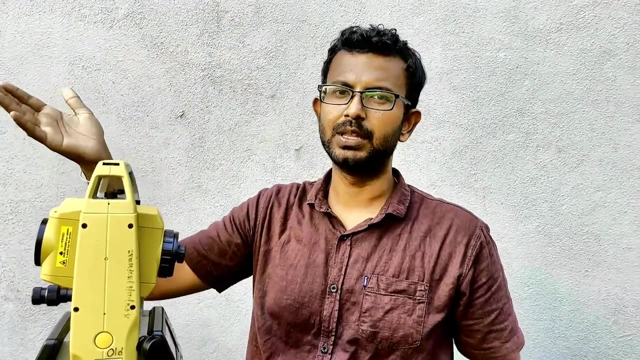 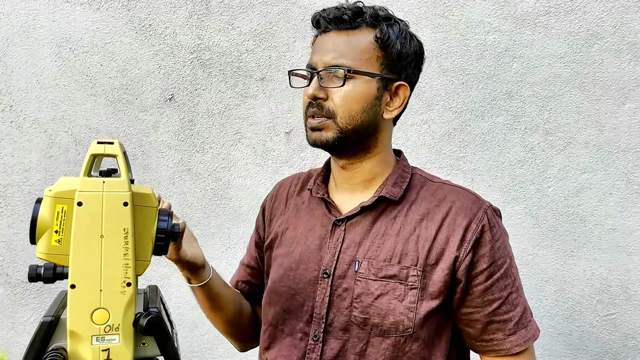 if the, if the instrument is made perfectly right without any instrumental errors, the face right reading should be exactly 185. because the face left reading is 5, there should be only 180 degrees difference between the face left and right. but since it is not perfectly made, 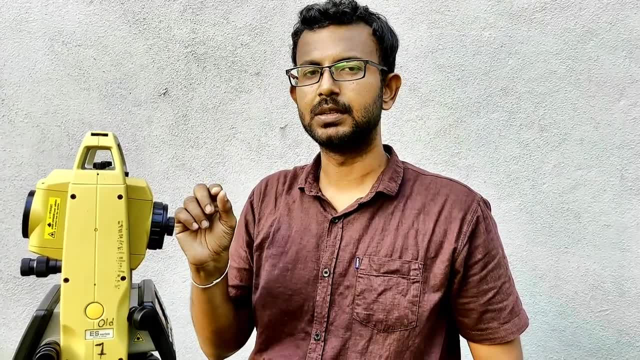 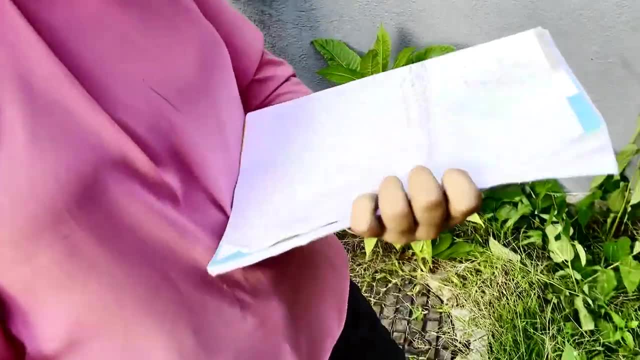 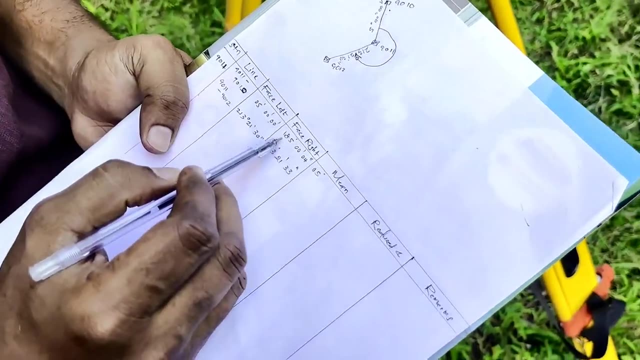 right. there's a slight error of 4 seconds, right, so we need to record these and get the average for the mean of these angles right. this is how we are doing it now. we know that this is 5. this is 185 0, 4. so even though this is this is 185, we know that. 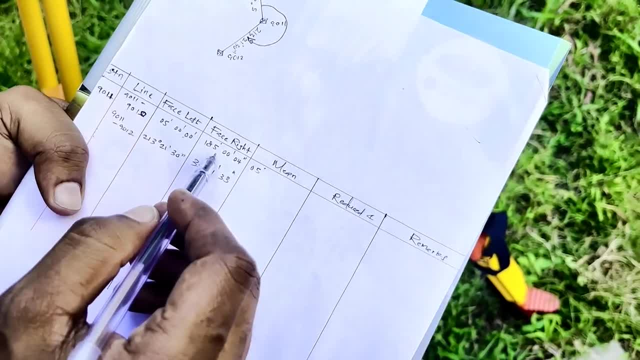 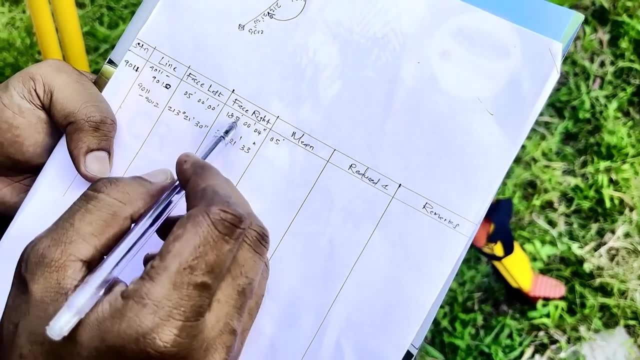 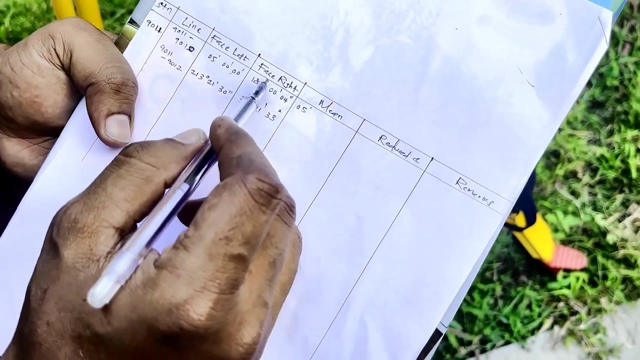 the 185 has come because we transit the telescope about rhodian axis. therefore, the difference between the face left and right is 180. right, in that case, we can reduce that 180 which was added to the face right reading from this face right reading, so we can reduce that 180 which was added. 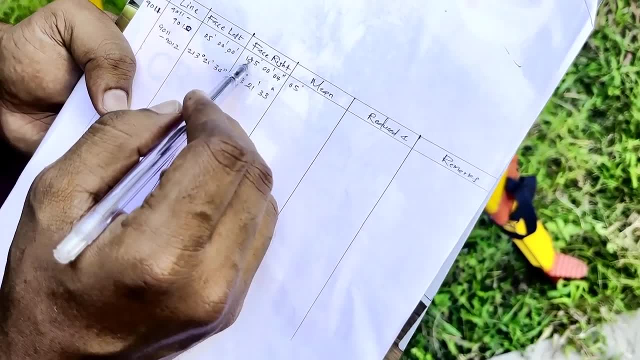 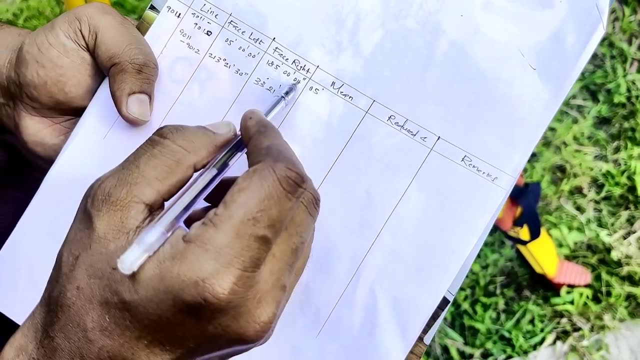 to the face right reading and then get the mean right. so when we deduct 180 from this face right reading, it is one. it is 5 0, 4. here we have 5 0, 0 right, so we have to get the average of 5 0, 0 and. 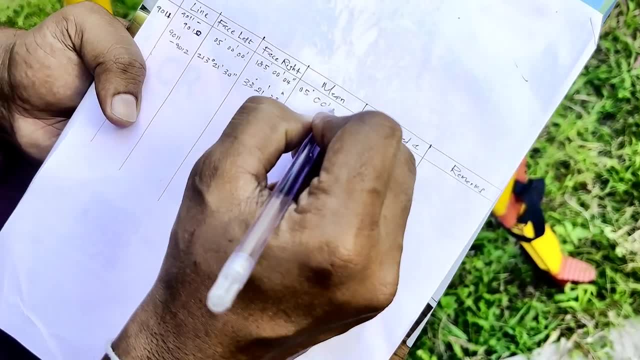 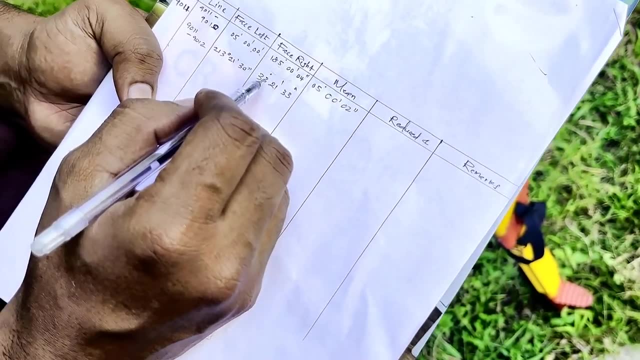 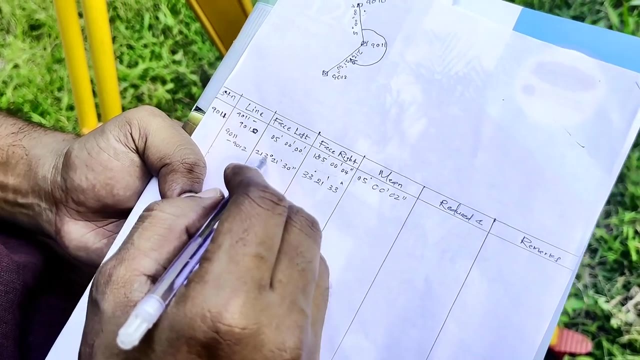 5 0, 4. right, it is 0 5 0, 2 seconds. right, that is the mean. he also liked that here, even though it is mentioned 33, this is: this has has the reading of 180 greater than this 230. so when we add the 180, it has turned 360 full circle. 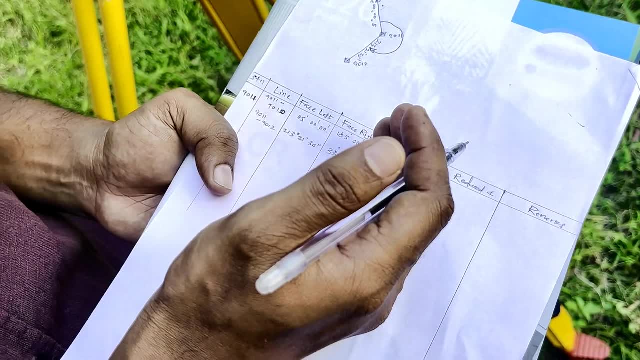 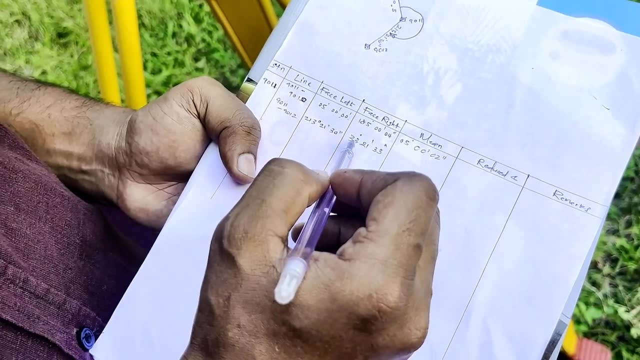 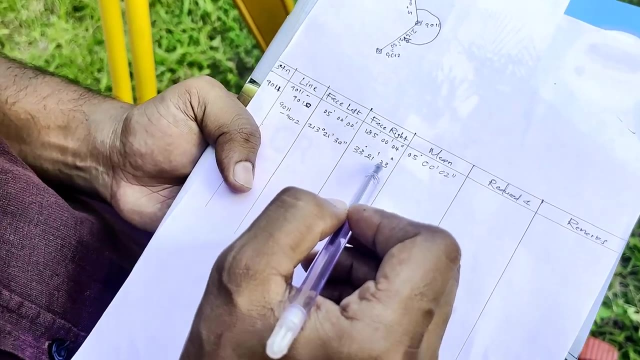 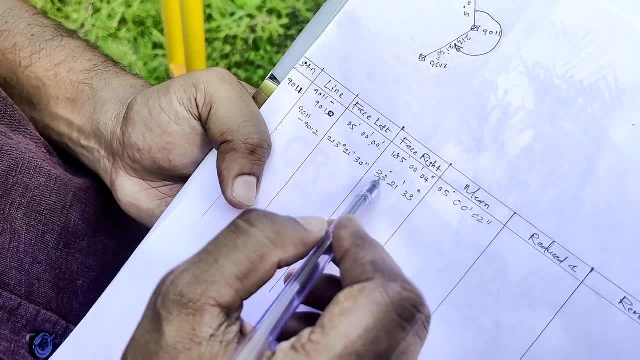 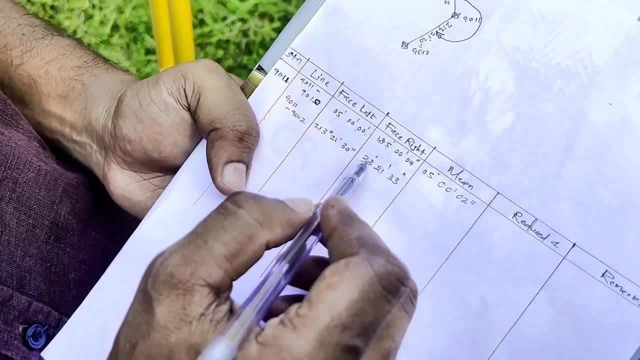 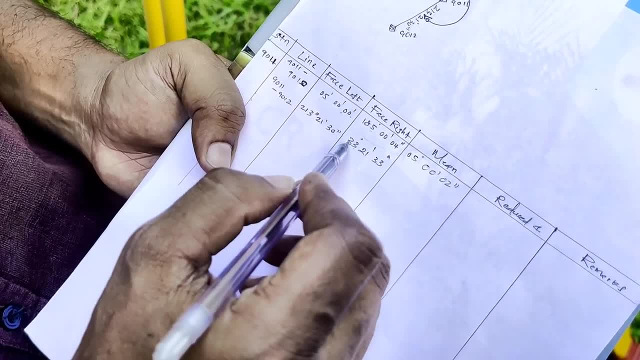 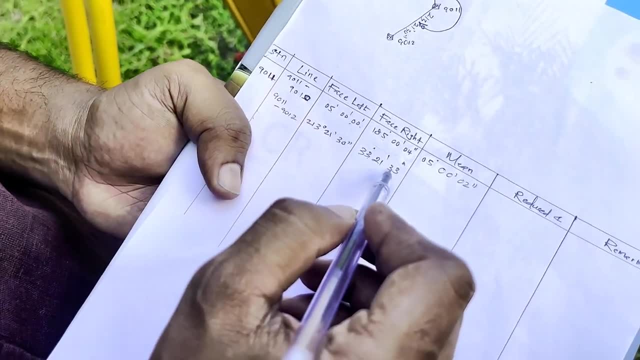 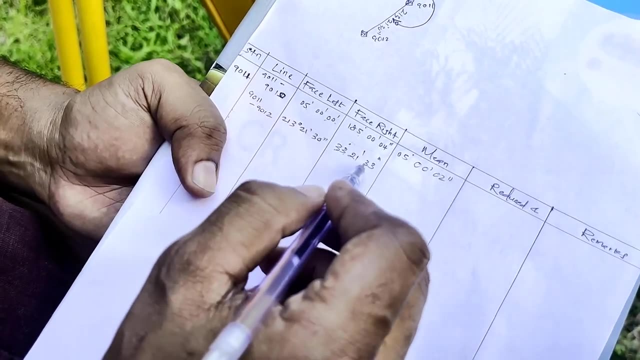 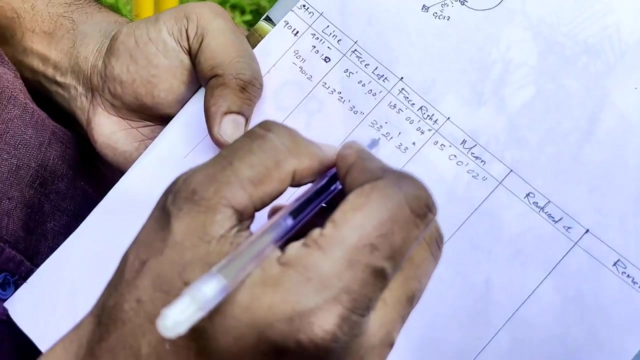 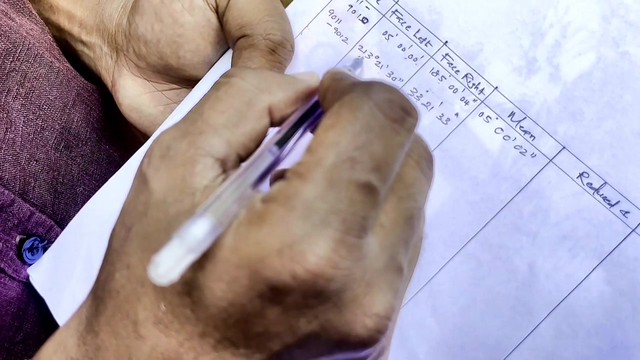 from- sorry, 180 from 393 21, 33 seconds. right, when you deduct 180 from 393 21, 33 seconds, the answer is 213 21- 33. so here we have 213 21- 30. right, the average between the mean value. 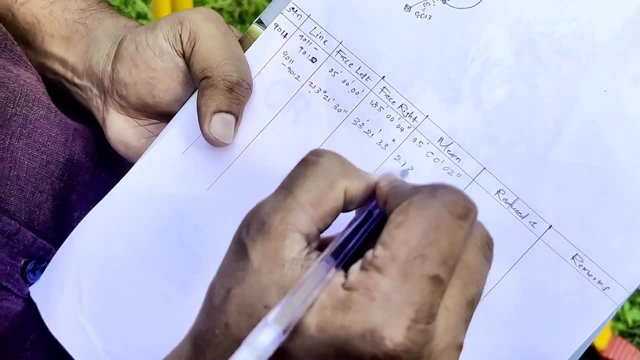 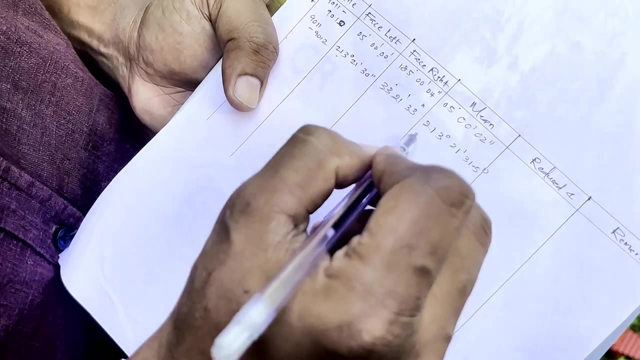 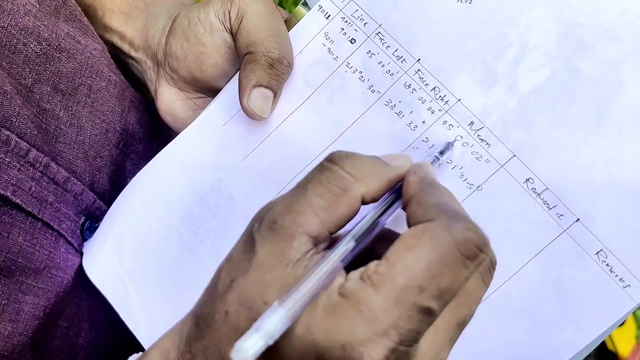 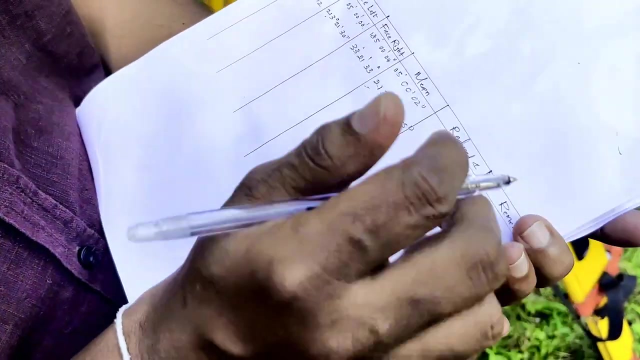 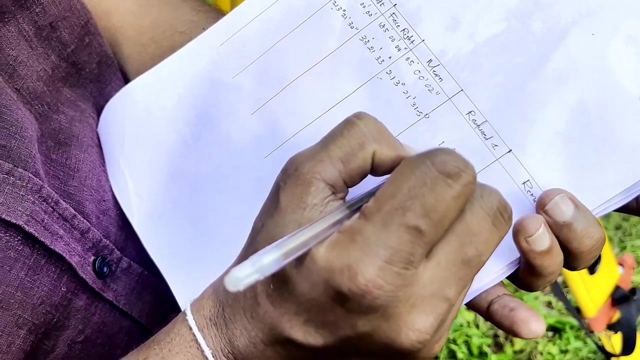 of these two value is 213, 21, 31.5 seconds, right, so, then, the reduce angle should be: we need to deduct this five, five degrees, zero minutes and two seconds from this value, right? so it is just like 29.5 seconds and 19 minutes, and. 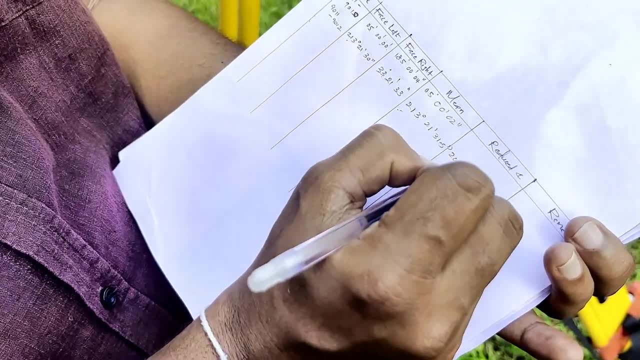 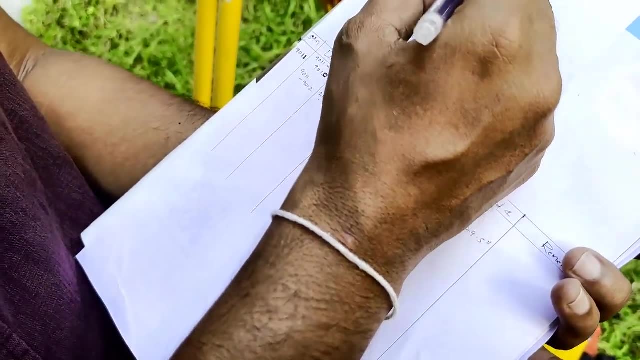 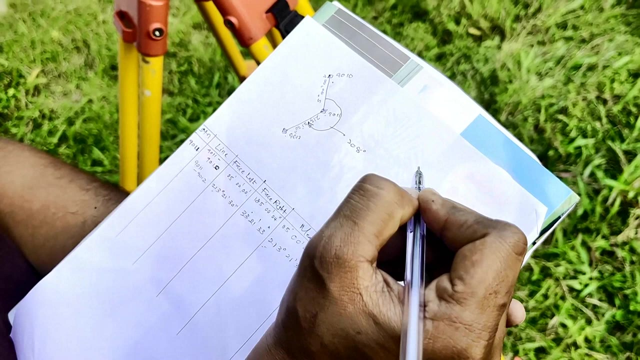 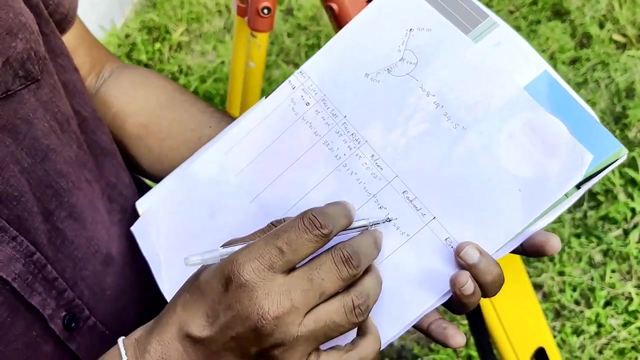 208 degrees. that is the included angle between 9010 and 9012. measured from 9011, this angle is 208, 19, 29.5. right, that is how we get this. the next thing is in the traverse. we need to get the distance. now you know that this is a control line. 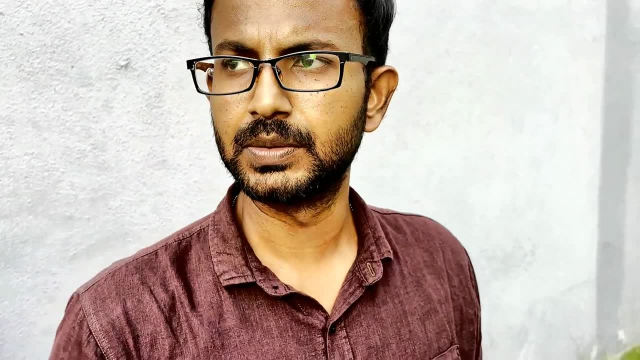 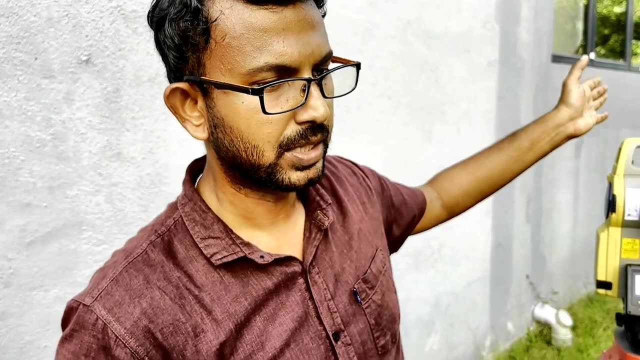 therefore, we don't need to get the distance here, because we have coordinates. we can calculate the distance using pythagoras theorem, right, but in this line, let's assume that this is not a control line. this is somewhere. this is a traverse, traverse station. in that case, we need to find out the 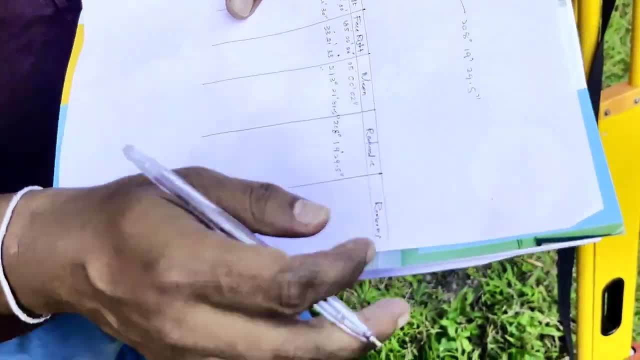 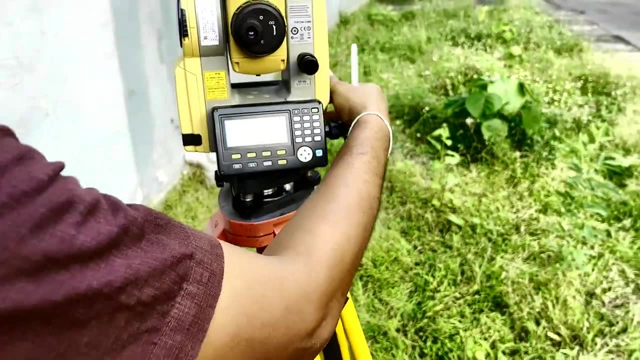 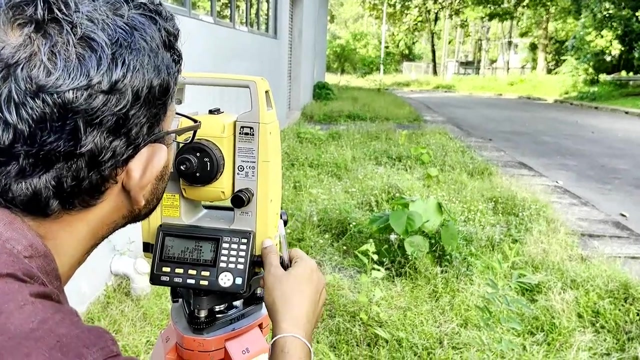 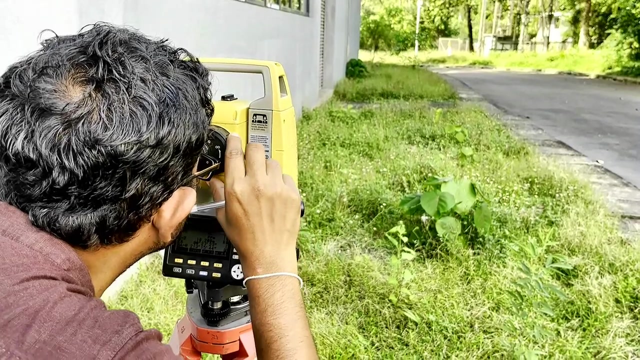 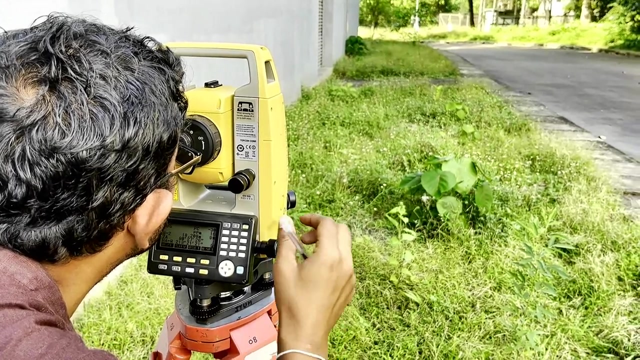 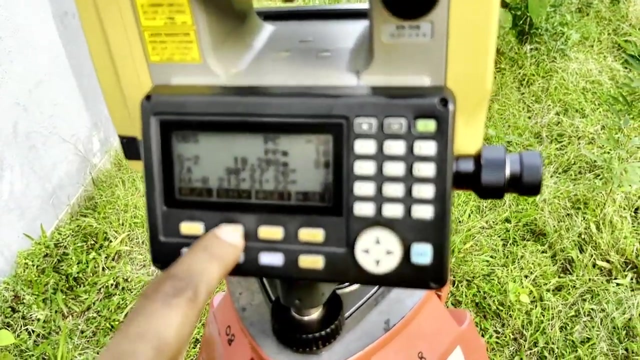 distance from 9000 11 to 9000 right for that again i'm i'm going to use- i prefer to use space left for distance measurement, So I target back to the 9012 and focus us perfectly. and now I need to measure the distance right so that I can use a measure. 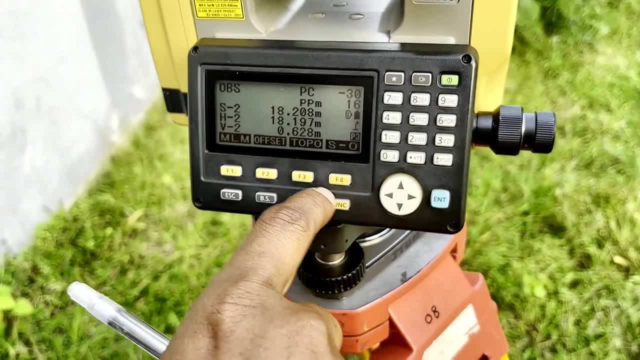 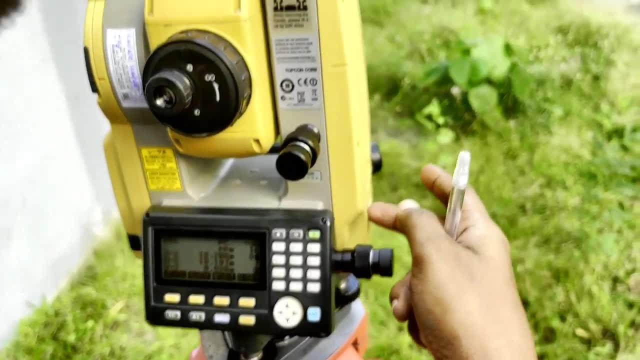 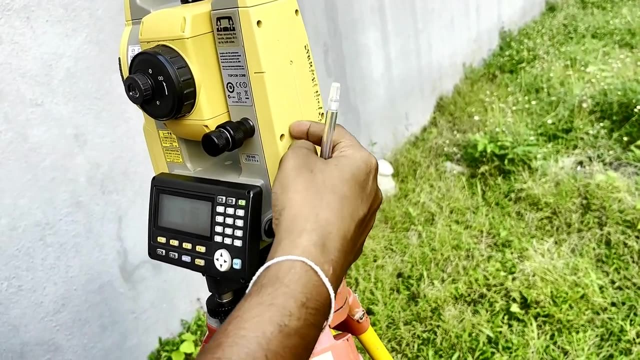 option here. if there is measure, I'll try to find out measure here. but measure is not there, In that case I can use this button. right, This is called the toggle key. right, if i press this button in this total station. right, this is called top cone. 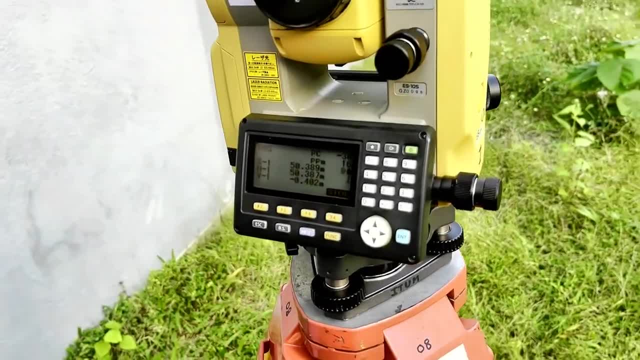 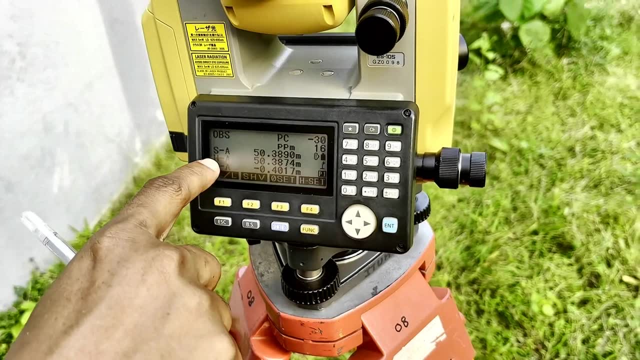 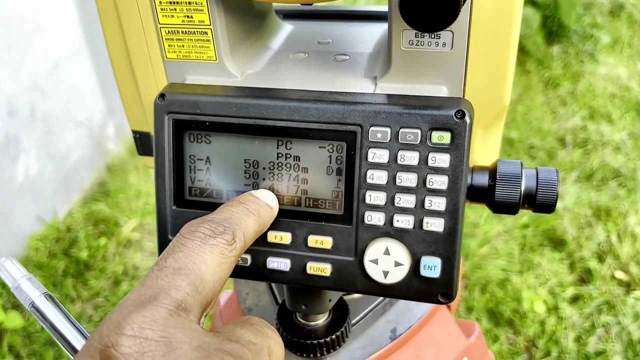 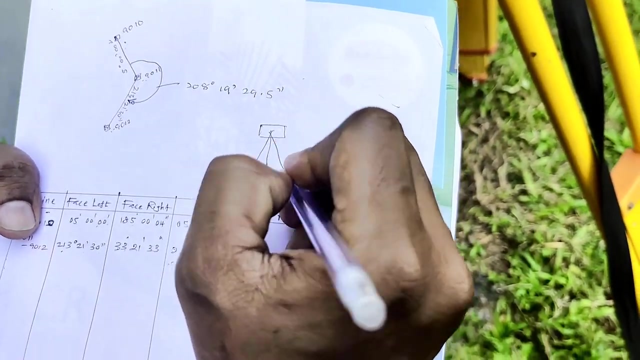 this top cone model. right, if i press this one automatically, the distance will come right now. you see the sa. the slope distance is 50.389, the horizontal distance is 50.387. vertical difference is 0.4017. right, this is just like this. now i have set the total station here and this is my prism. 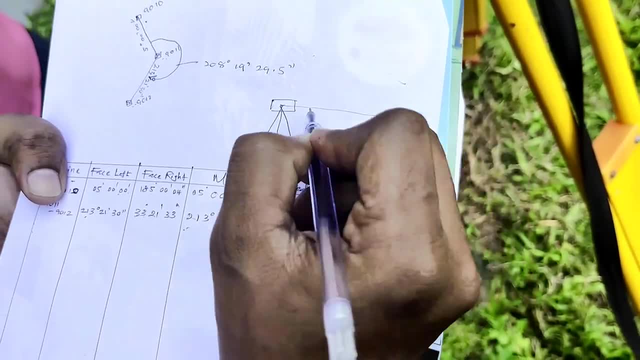 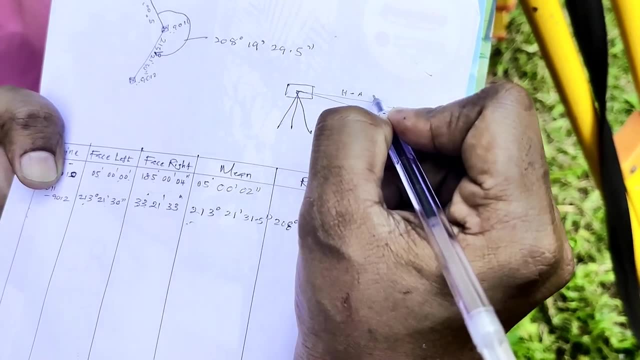 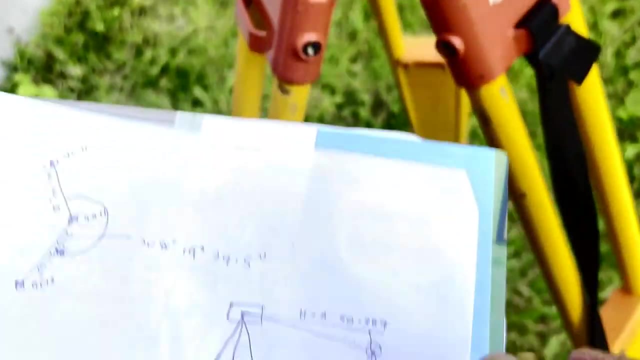 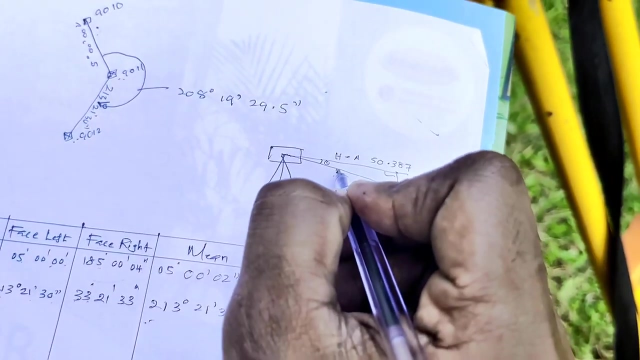 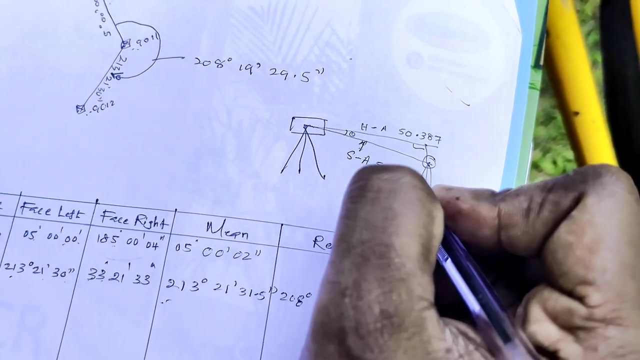 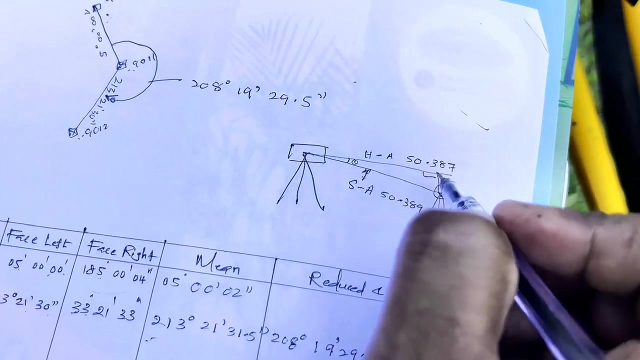 somewhere there, right, this is this. this is hd o, h a right, h is 50.387, right and sa. that means slope, slope distance. the sa is 50.389. now, you, you know, always, this slope angle is greater than the horizontal distance in a right angle, triangle, right, and this is minus. minus means from this level you have. 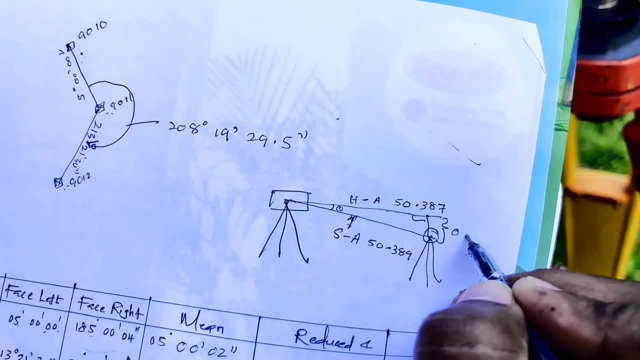 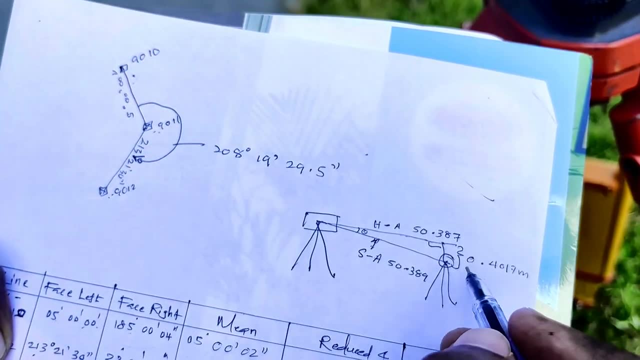 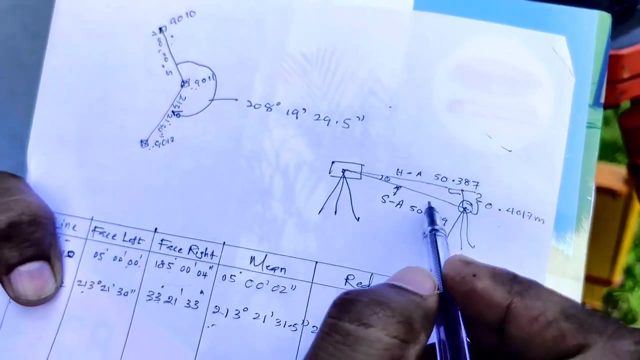 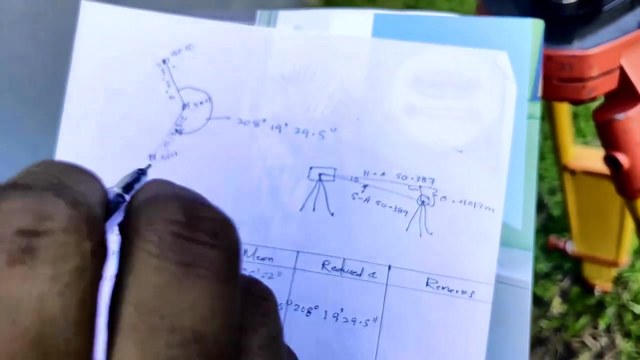 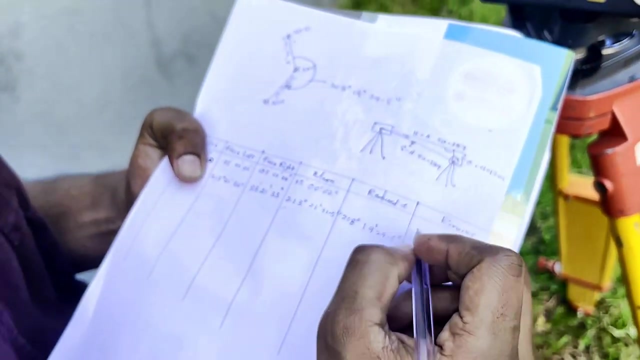 the vertical difference of 0.4017 meters right, one, seven meters from the level of the horizontal axis of in of the telescope and between the axis of the target prism right. so that is the meaning of that. but here for the traversing we are only going to record this horizontal it. horizontal distance, h a right. 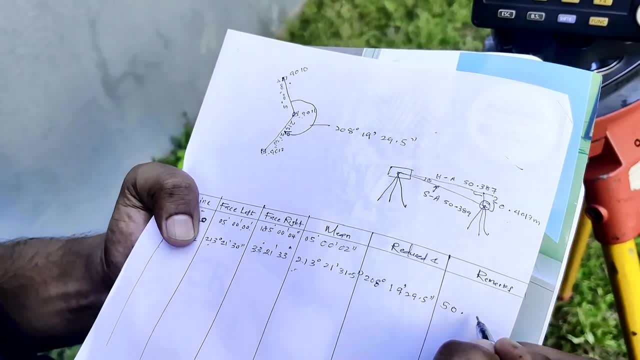 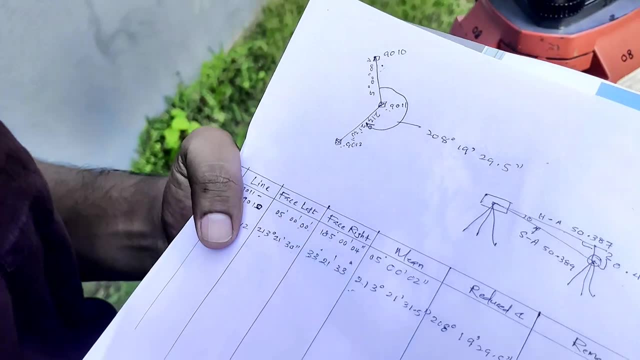 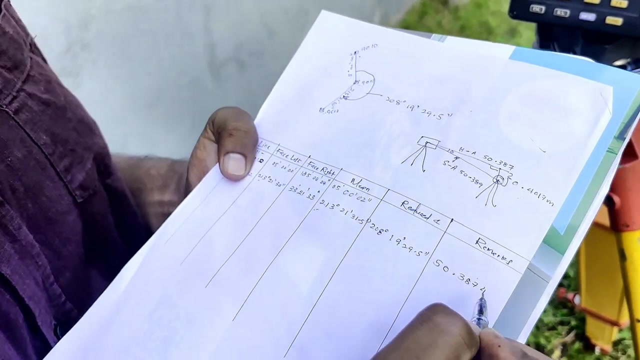 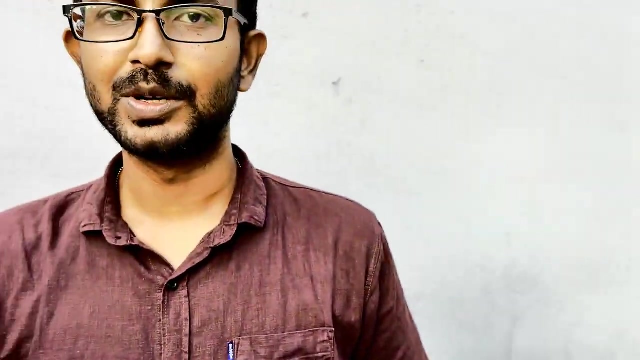 and sa here. we know that you only have to clear the top of that hill and this is the see or and sa. we always find that our drop point is at 50.387, so it is better to the third decimal point right now, today. now you learned how to do the traversing. 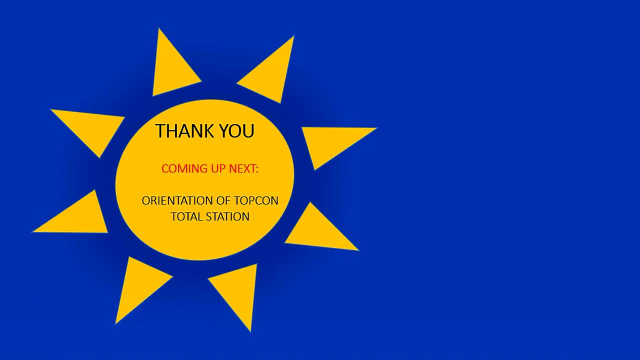 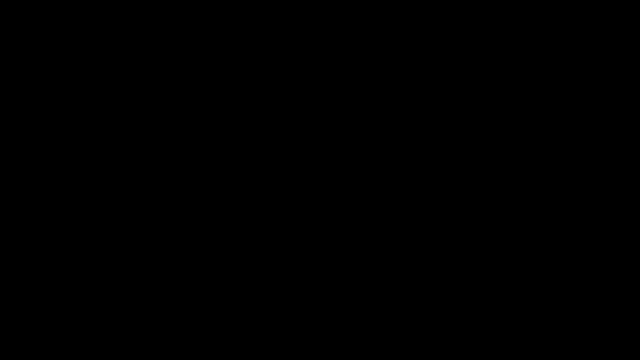 this video coming up next is orientation of a total station. don't forget to subscribe this channel and click the bell button for more of the very latest videos. you.